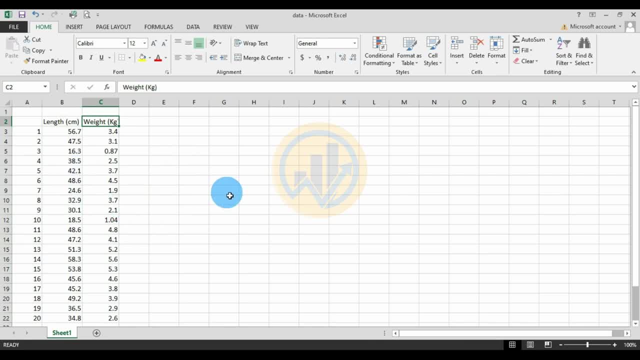 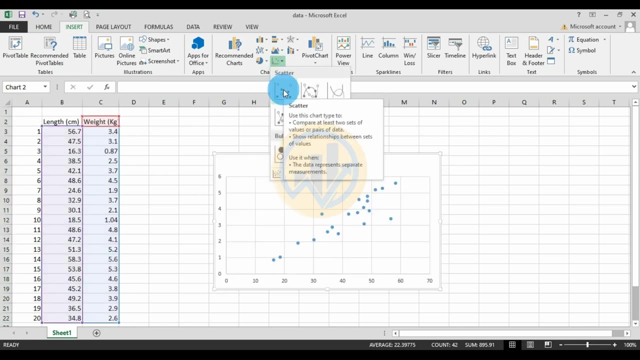 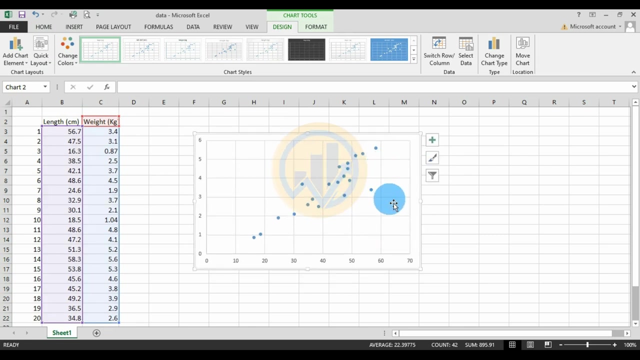 Okay, this data analyzer for the first of the linear regressions. They select the data- fish and fish length and weight, the data selected and go to the insert menu and select the chart menu. Select the scatterplot, Click the OK button. Then create the scatterplot. Okay, delete the title, Select the center part of the line, Go to the format menu and click the. 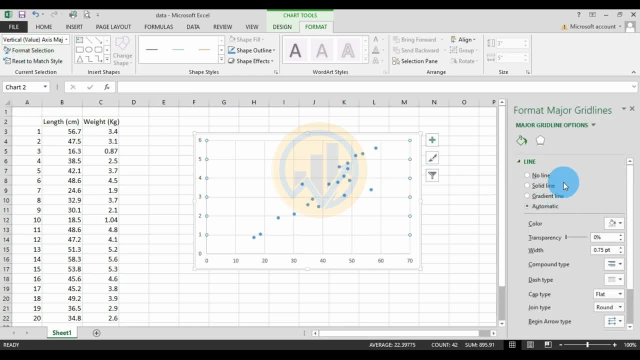 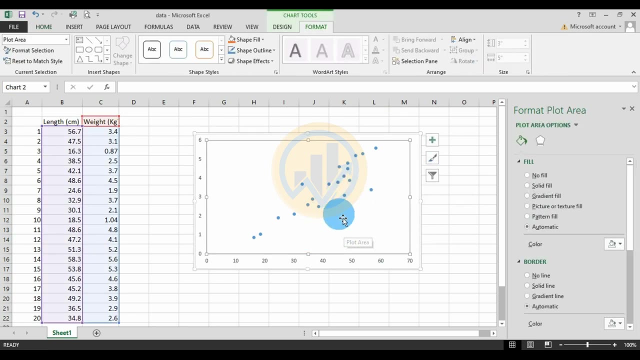 format selection. Open the new tab for the format. manage guidelines: The guidelines: the no line: Okay. select the horizontal value: The no line: Okay. select the chart. Change the color: Background colors: black, white, Okay. select the line. 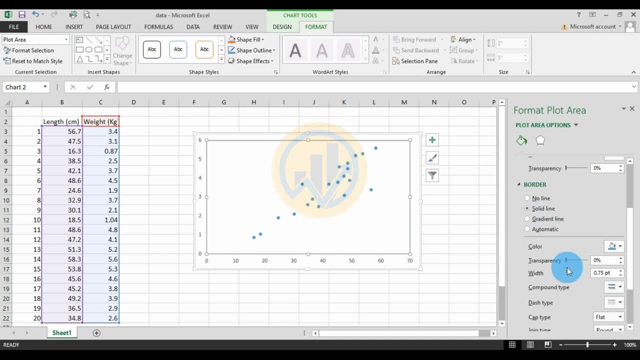 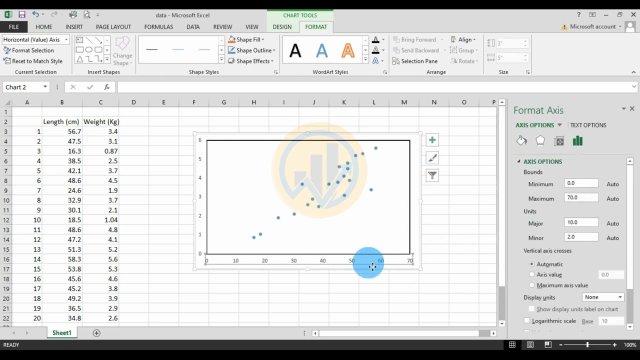 This is the border. Select the line color for the black: Okay. increase the width for 1.5.. Okay. Next select for the exceeds the value. Change for the font Time: how many: 10.. And theата access. 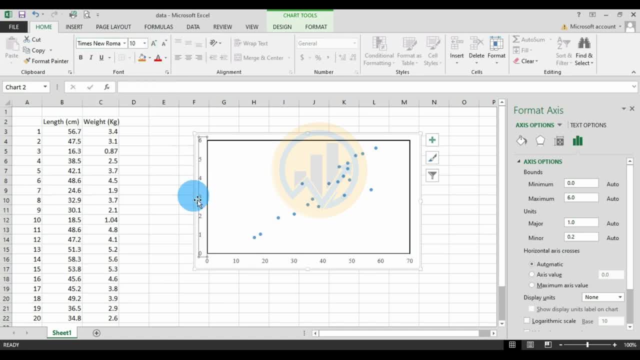 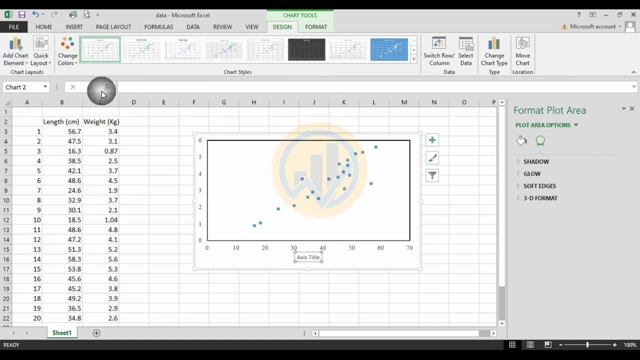 the font. Change the font, change time movement and increase the font 10. okay, add the y axis and axis title. select the graph, go to the designing and they add a chart element axis title for the primary horizontal and add to the next one for the. 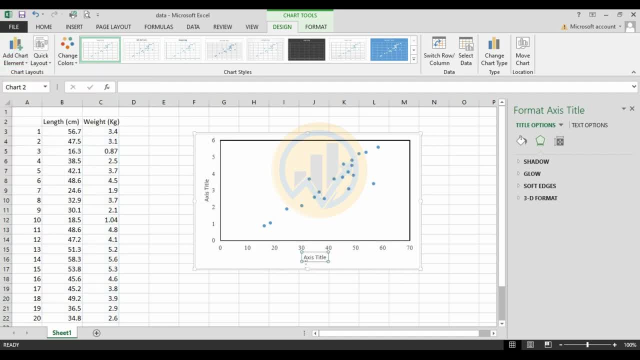 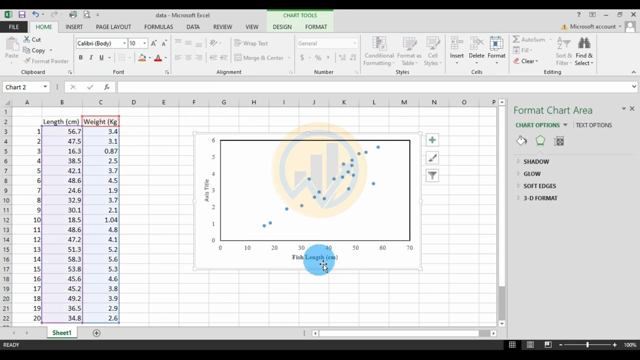 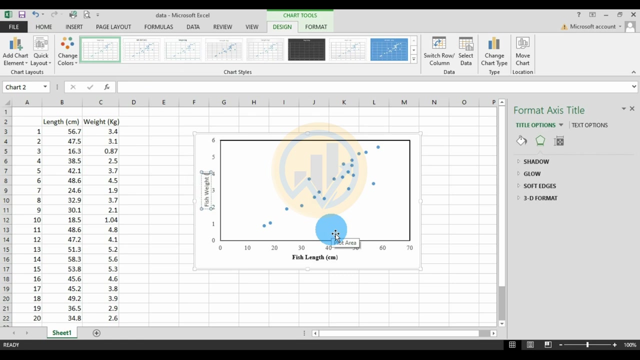 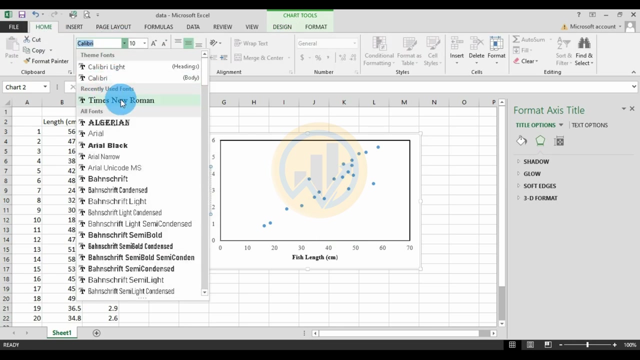 vertical: okay, the horizontal type. for the fist length: face length, the unit centimeter: okay, select and the change the font. click the bold. okay the color. change the black. okay, the next one. for the y axis: title: face weight: the kg. go to the home menu. change the font and the black with the gold: okay. next the 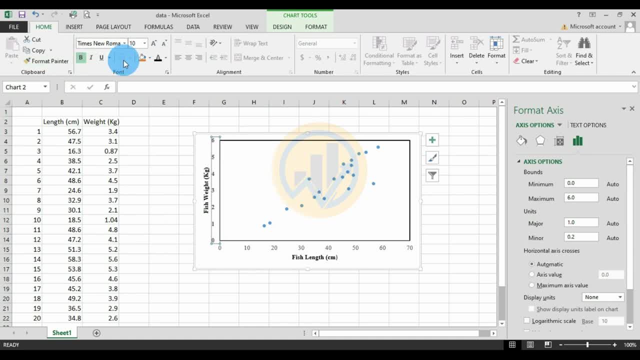 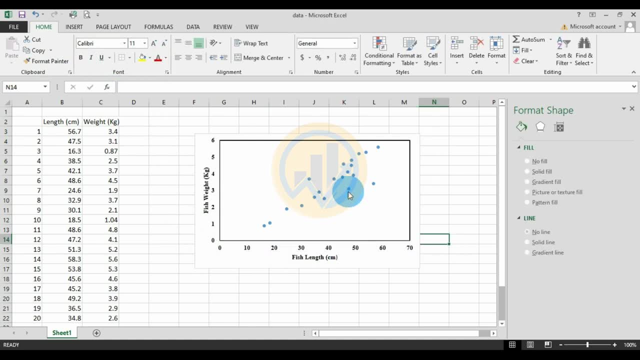 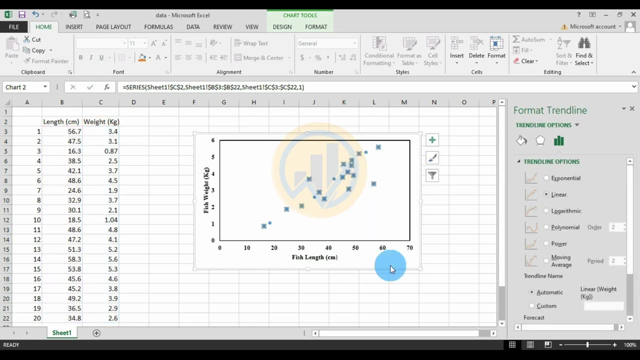 value change bold and black. the next y axis value: change the black and bold. okay. next click for the value right. click the button and they add the timeline. the open new tab for the options in the linear regression. select the linear regression and the rolling the mouse, the. select for the display equation, the on. 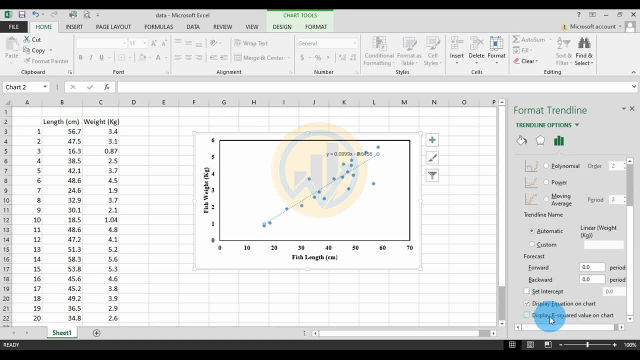 chart. the next one check box for the display R square value on the chart. okay, this is for the linear regression in the fish data. okay, select the data. the change the font, increase it to all and the black. they click the bold next to select for the timeline. okay, they. 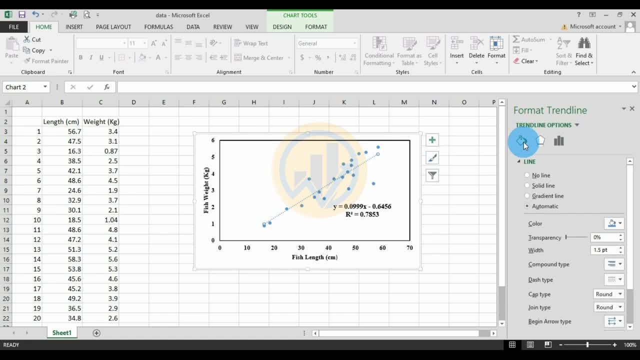 select the timeline and use. for the color bucket: change for the color black: increase the water. the width: 1.5 and the line: the dash type. for the straight line: okay, select the straight line, the next one for the color change. for the the simple: okay, the change to. 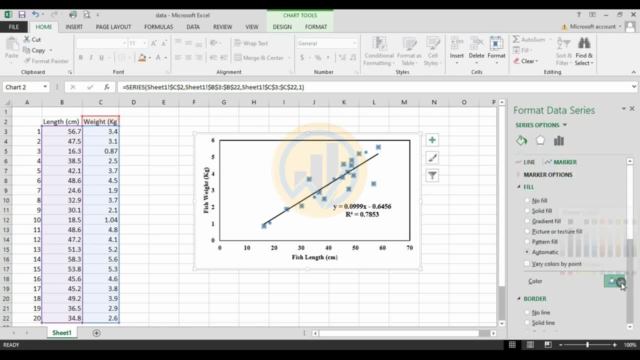 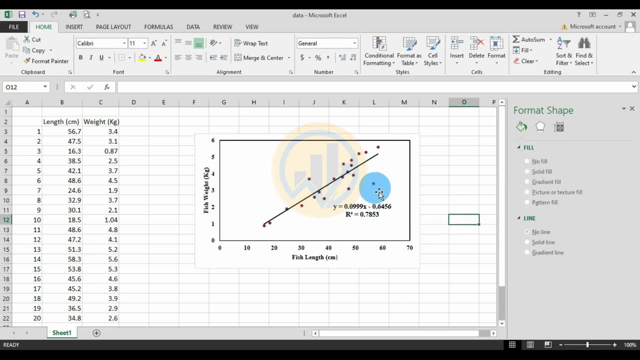 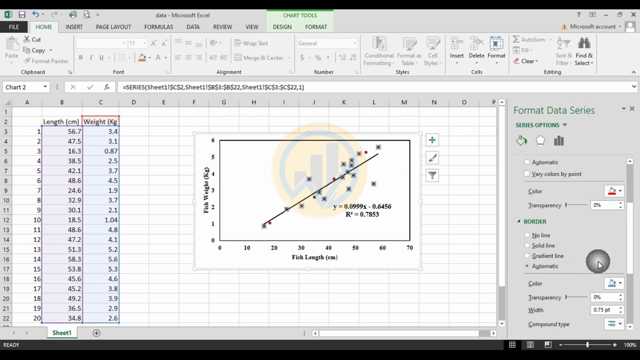 the marker. the change to the color blue. any other color is selected. I select the red color, okay, or any other color. dark red to the border under the color to the dead: okay, okay, this is for the linear regular sense in the EXELS are softer. next one: 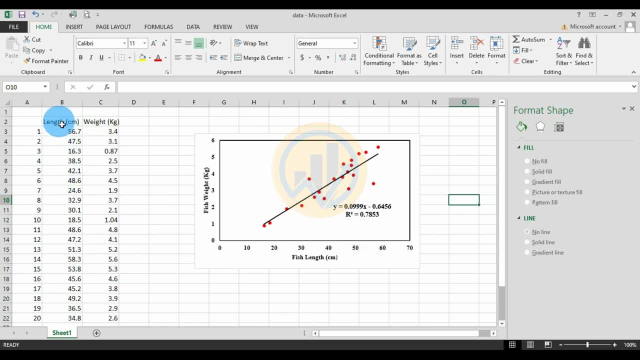 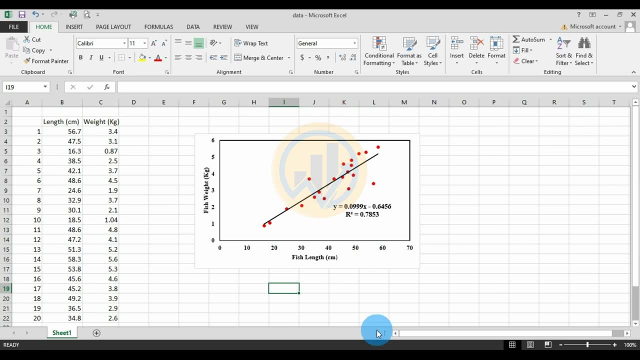 the, unless it for the correlation: the fish length and weight data. okay, the one of the shortcut method, the correlation for the this data correlations equal the formula for the CO or a EL coral. enter the: select the value. okay, the end of the comma. the next one, the value, the next to the complete the bracket. okay, click the. 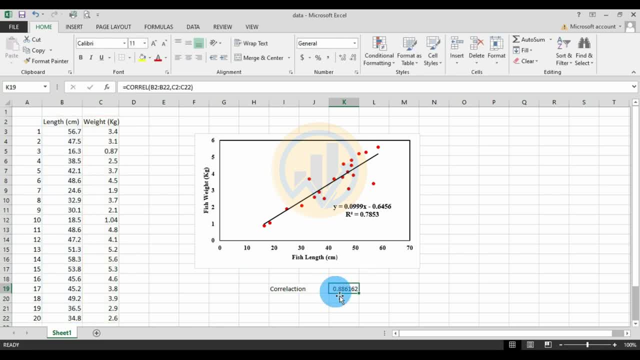 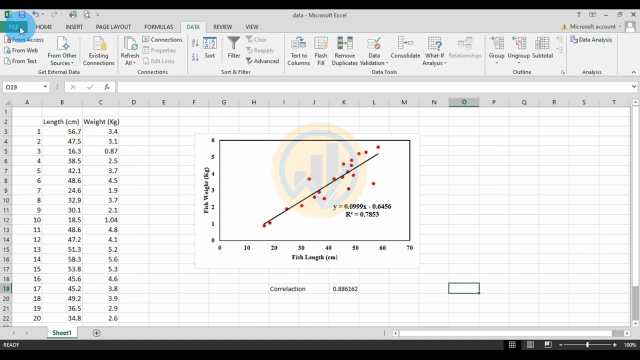 enter. this is for the correlation in the piece length and weight data. okay, the next another method for the correlation method: go to the data menu that analyzed the data on laser tool, the how to active this tool. go to the file menu and go to the options menu. open the new tab and go to the 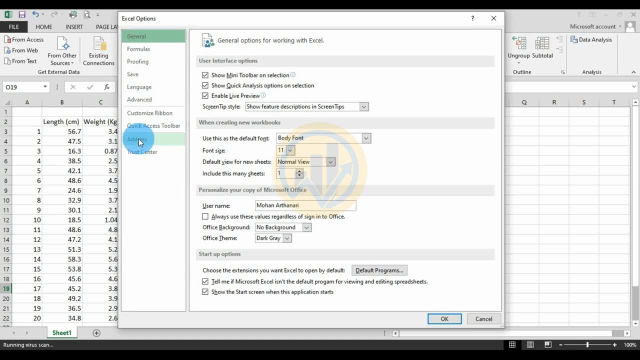 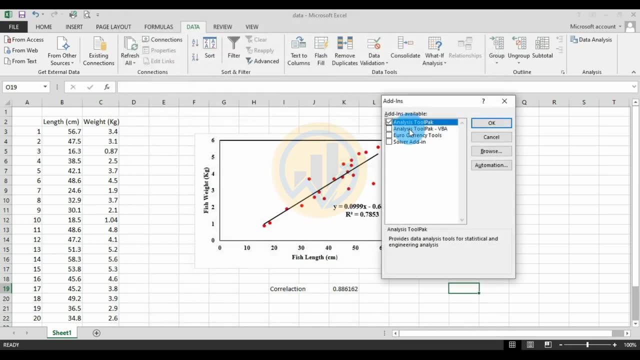 add-on: okay. go to the manage the excel add-on line. okay, select the excel add-on line, go to get it. the button click and the click tick box, check box for the un unlike tool pic. then click OK. then active this wet analysis tool. then click the data analysis tool, select for the correlation you know and click the. 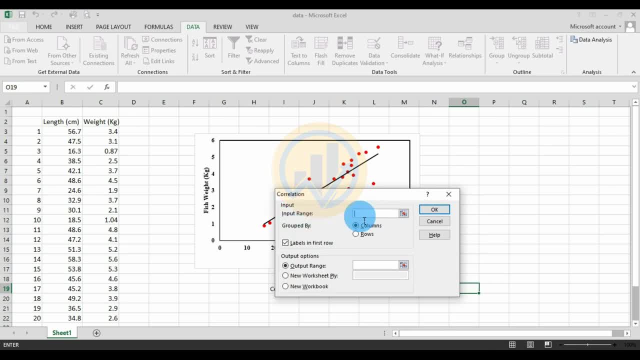 ok button. the open the new tab for the input ranges. enter the value, so select the data analysis tool. select the data analysis and click the quis Thunder. select this button. then select the value for the fish length and weight. then click the ok button. the grouped by the. now the enter the data for the column format, so click the.